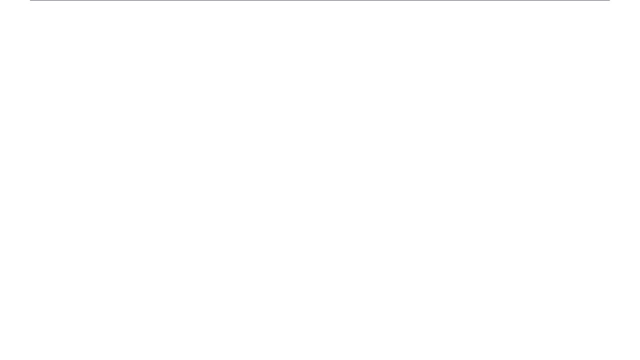 of single variables or, better still, functions of only one variable, and that was usually represented as we had: y equals f of x. Now the function here, y, is said to be a function of only one variable, and the variable in question is the variable x. So this is a function, a function. 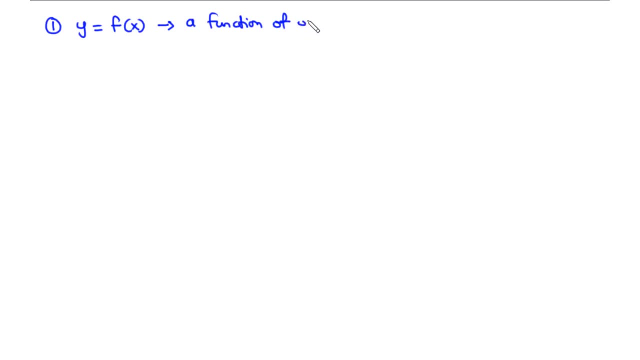 of only one variable or a function of a single variable bị tunes, and that is the variable x. Now what this primarily means is that the function takes in a single x input to produce a single y output. so an example of such a function we can be looking here: X1.. 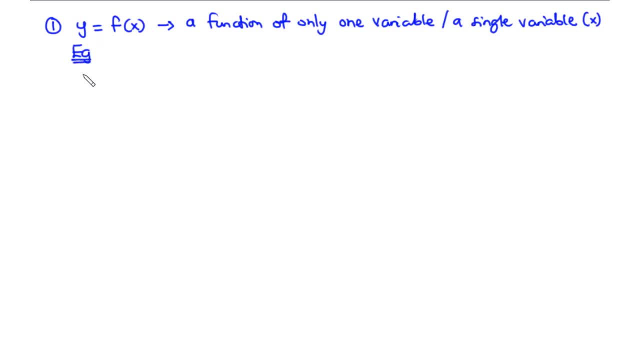 looking at the equation of a straight line. So let's say we have an equation: y equals 5x plus 2.. So this is said to be a function of only one variable, because it requires a single x input to produce its corresponding y output. So this is an example of a function. 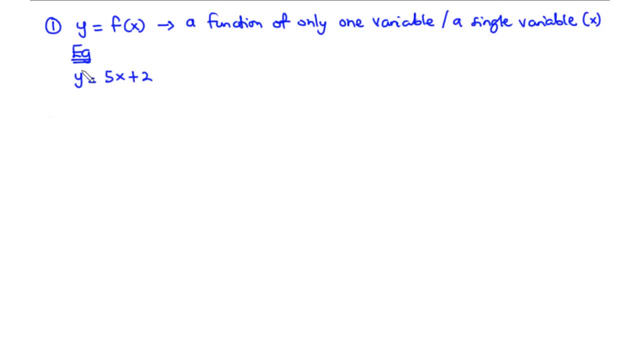 of only one variable. Now, moving away from this, that is, functions of single variables, let's focus on functions of several variables. functions of several variables, So functions of several variables, on the other hand, take in multiple inputs, that is, more than one input. 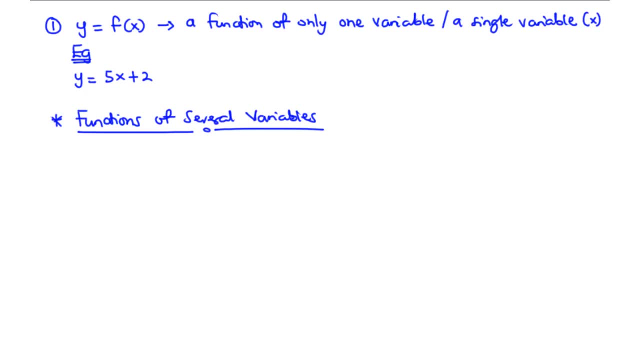 to produce either a single output or multiple outputs. Now we can consider the function that is given, as z equals 5x plus 2.. f of x, y. Now this is a function of two variables: x, and then y is a function of two. 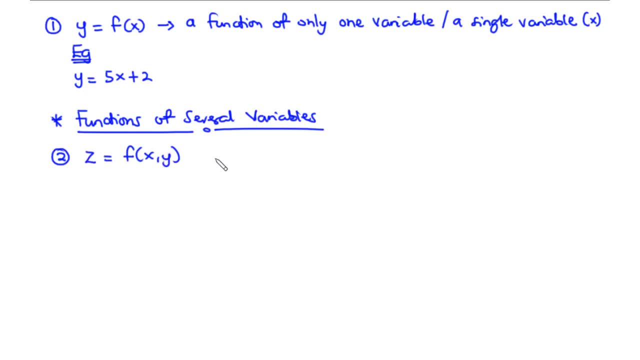 variables, which produces a single output value: z. So this is a function, a function of two variables, two variables, And these variables are x, y. These are the two variables, x and y. So an example of such a function, we can talk. 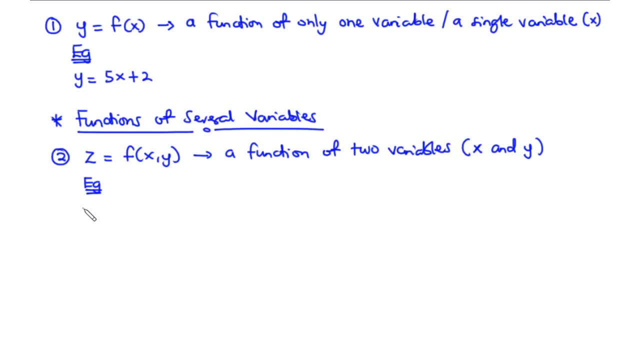 of the function that describes the area of a rectangle and that is given by a equals the length times the width. This is a function of two variables and it depends on. it depends on the variables, the variables l and w, the length and the width. 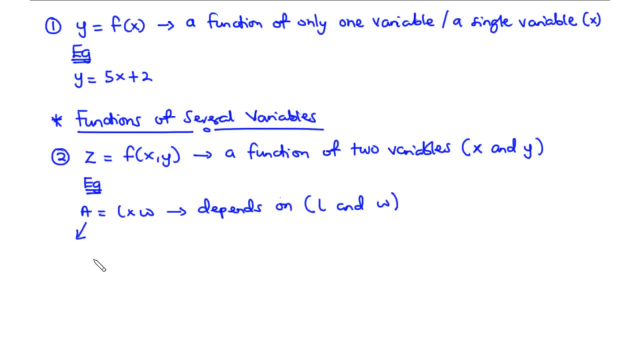 Now we can represent this in the functional notation form as f of l, w, and that is equal to l times w. So this is a function of two variables. It depends on the length of the rectangle as well as the width of the rectangle. So for functions of n variables, let's say: 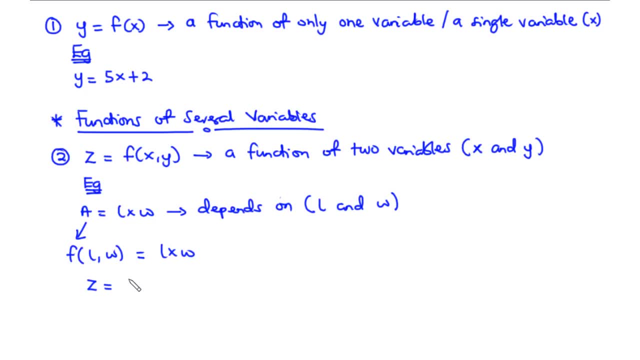 functions of, in this case, two variables: z equals f of x, y, Okay, Okay, Okay, Okay. z is said to be the dependent variable, dependent variable, And then x and then y are said to be the independent, independent variables. These are the independent variables. What? 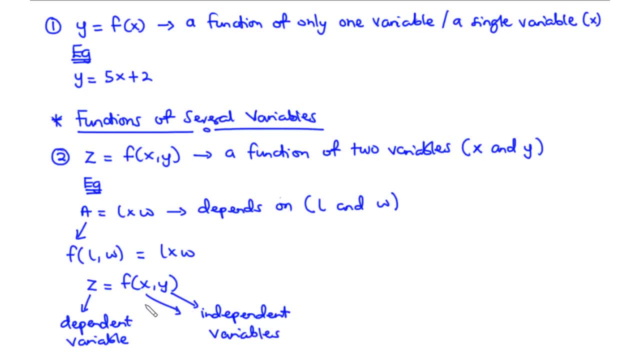 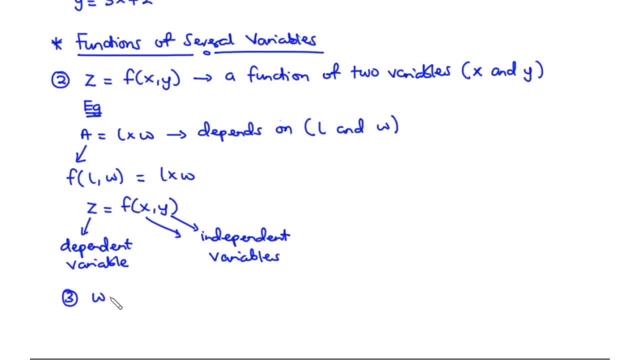 this primarily means is that z depends on the values of x and then y, So x and y are said to be the input values and then z is said to be the output value. now we can also have a function that looks like this, that is, w equals f of x comma y comma z, and this is said: 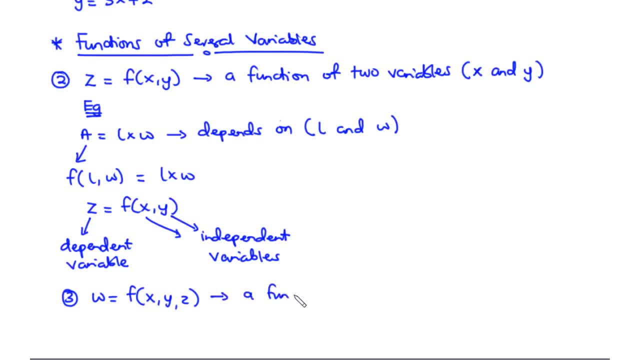 to be a function, a function of three variables. a function of three variables: it depends on the variables x, y and z. an example of functions of three variables: we can have the function that describes the volume of a rectangular box. so the volume of a rectangular box is given by 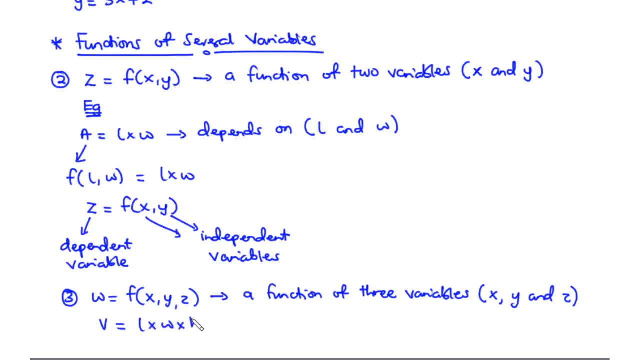 the, the, the length times the width times the height. so we have this in the functional notation form as f of l comma, w, comma h, and that is equal to the length times the width times the height. so this is a function of three variables. so usually you'll be asked to find either the: 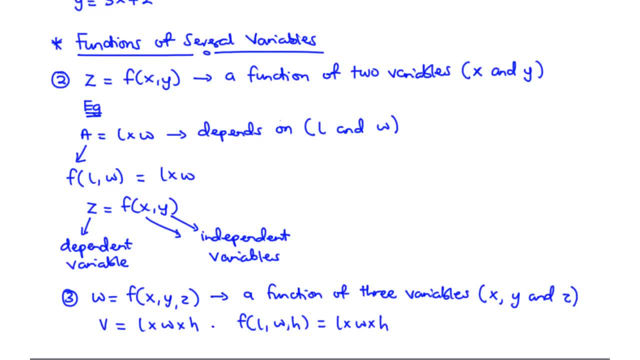 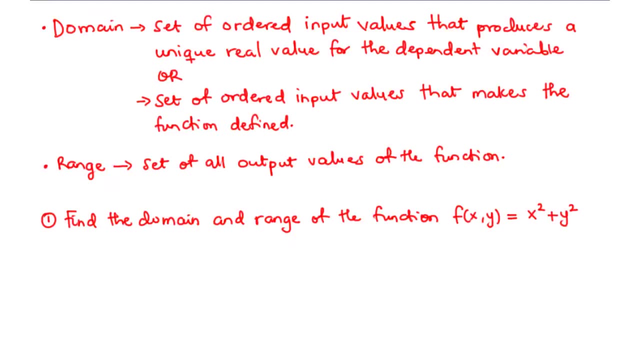 domain, or the range of a given function. now what you need to understand here is that the independent variables of any function may be restricted to lie in some set d, and this set is called the domain of the function. so let's look at what the domain actually means. so the domain: 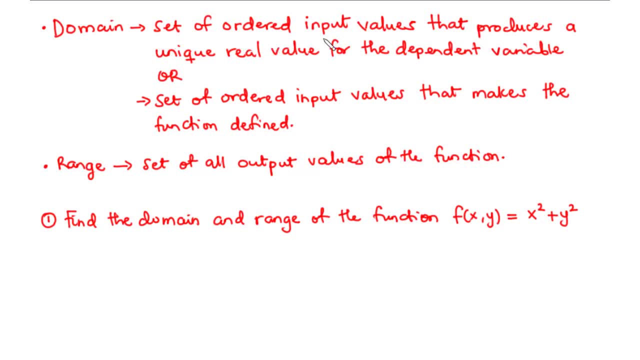 of a function is nothing but the set of ordered input values that produces a unique real value for the dependent variable. so it is the set of ordered input values that produces a unique real value for the dependent variable, or we can have the domain to be the set of ordered input values that makes the function defined the 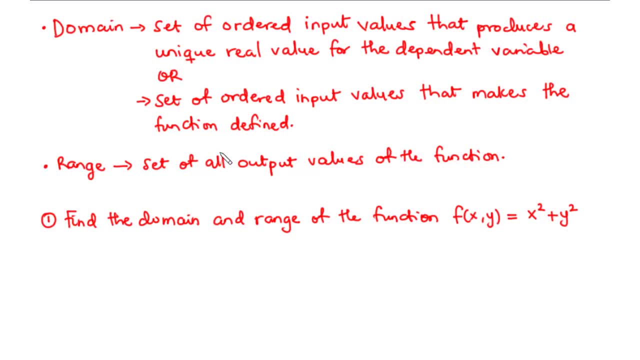 set of ordered input values that makes the function defined, and as well we have the range to be the set of all output values of the function. so the domain focuses on the input values. that's going to make the function defined, that's going to make the function meaningful, and then the range. 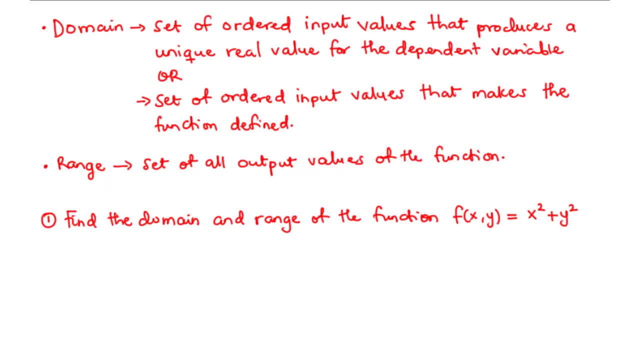 is focusing on the output values, the set of output values of the function. So here we have an example. That is example one. We are asked to find the domain and range of the function. f, comma, y equals x squared plus y squared. So let's try this example together. 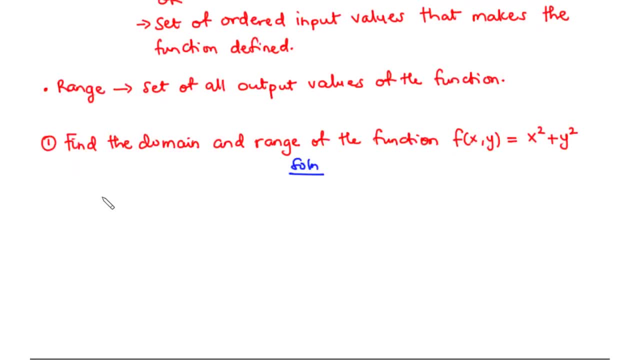 So we want to find the domain and range of this function. So first let's focus on the domain. How do we find the domain of this function? So we have the function f of x, y, and that is equal to x squared plus y squared. Now this is a polynomial function of two variables, x and y. This is a. 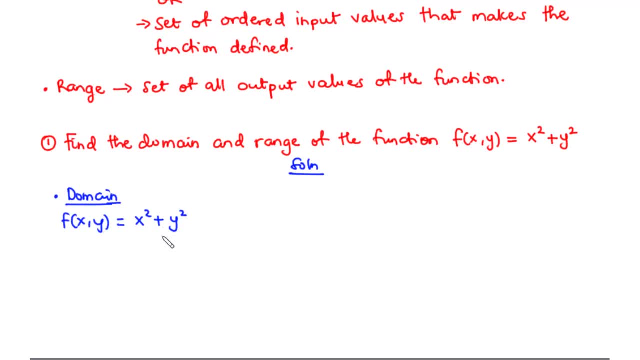 polynomial function of two variables And looking at this function, if you want to find the domain, that is, the set of ordered input values that makes the function defined, it means that we need to focus on the input value of the function. So we want to find the domain of the function f of x, y, 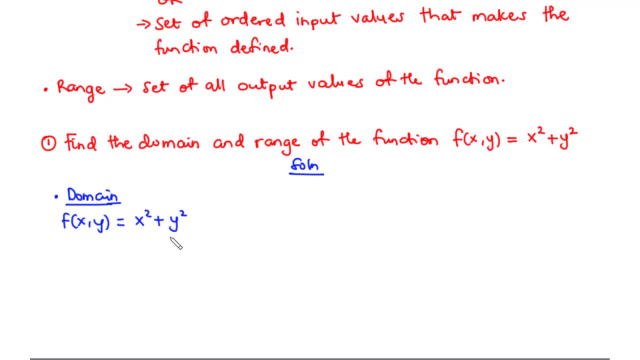 values and see for what input values are going to make this function defined. Now you realize that there is no restriction on the x or the y value. Now what this primarily means is that whatever value you are going to put in this function in place of x and y is going to make the function. 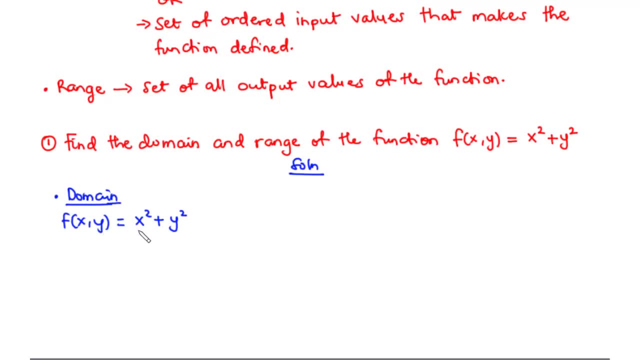 defined. Whichever values you place in this function in place of x and y, you are going to obtain a unique real value at the end. Therefore, we say that the domain of the function is the set of all ordered pairs, ie an particular set of all ordered pairs. 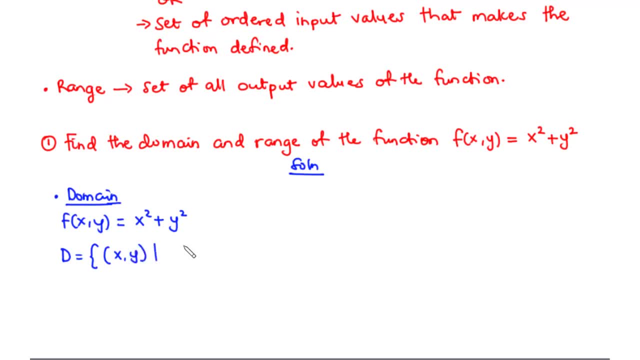 x comma y, such that x comma y is the set of all real numbers for a two-dimensional plane. Now notice that the domain of any two-variable function can be fit everything mismos. achive car function is the subset of the two-dimensional plane, Since there were no restrictions on 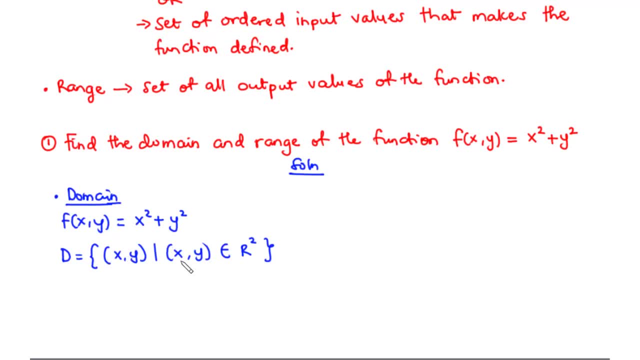 x and y. it means that the domain is actually the set of all ordered pairs in the two-dimensional plane. So this is how we write the domain of a function, So the set of all ordered pairs- x, y, such that that is the vertical bar. you can also replace that with two dots like this: 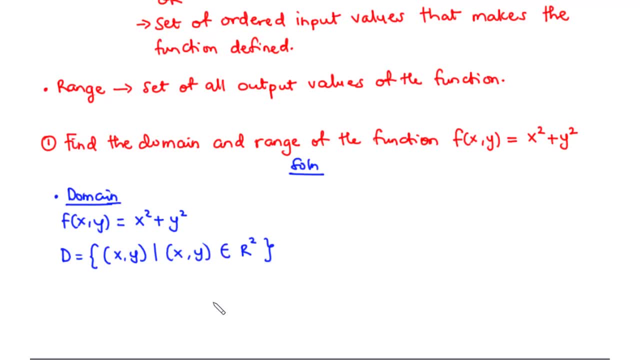 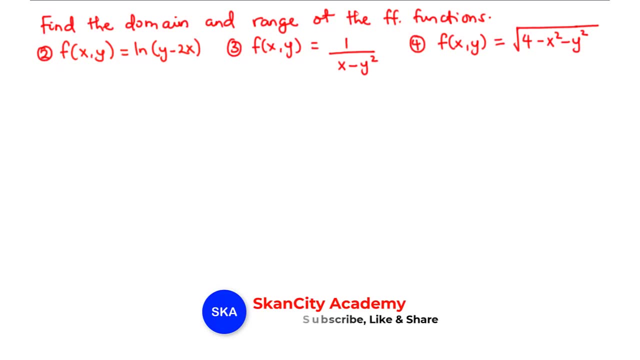 So such that x- y is the set of all row numbers in the two-dimensional plane. So we have a number of functions here. Let's try to find the domain and range of these functions. So we are going to start off with example two. So for example two, we have the function f of x y, f of x- y. 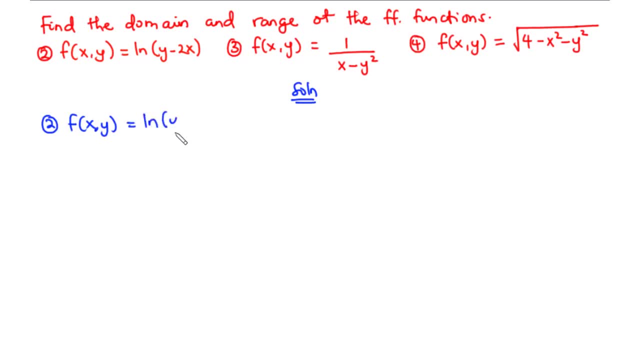 and that is equal to ln of y minus 2x. So this is a natural logarithmic function. Let's try to find the domain first of all of this function. So, talking about the domain, we want to look at the set of all ordered input values. that makes this function defined, The set of all ordered input. 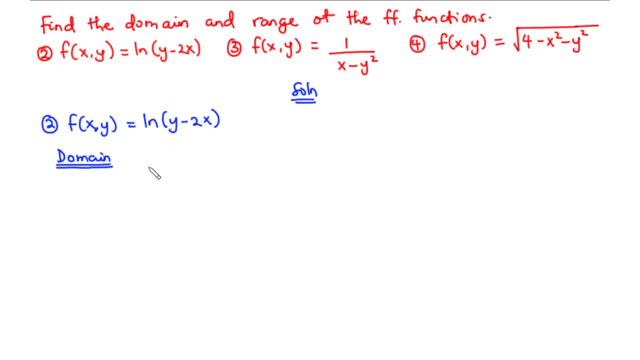 values. that makes the function defined. Now for a natural logarithmic function or for a logarithmic function. we know that the argument here should be greater than zero. Let's say, if we have ln, then for ln to be valid it means that p should be greater than zero. 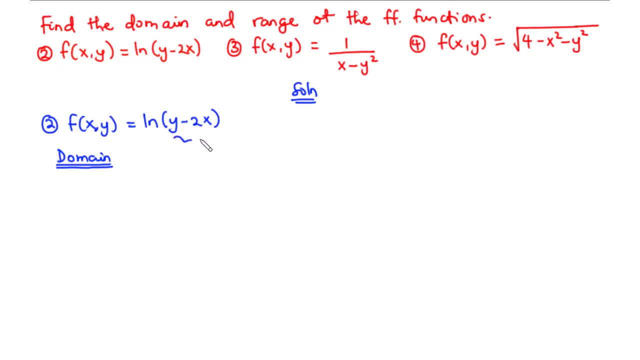 Therefore we are going to set this expression greater than zero, So we have y-2x greater than zero. we transpose negative 2x to the right hand side. we have y greater than 2x. So you realize that here we have a constraint. 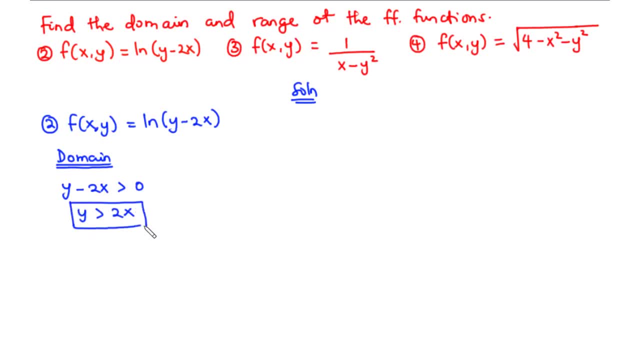 We have a constraint. let's say that we have a constraint, that we want to write with the a restriction. the restriction is that, for any value of x, y should be greater than twice of the value of x. so this is the restriction. we have, therefore, to find the domain. we say that the 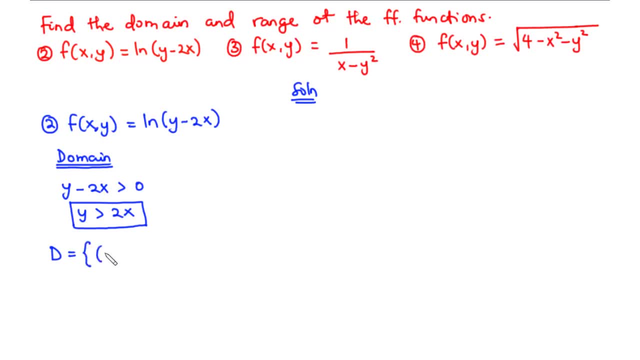 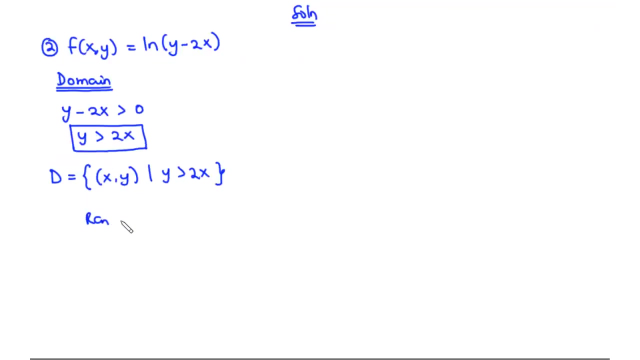 domain of this function is the set of all ordered pairs, x, comma, y, such that y is greater than 2x. this is the domain of the function. now to find the range, to find the range of this function. to find the range of this function, first, we are going to let z to be equal to ln of y minus 2x. 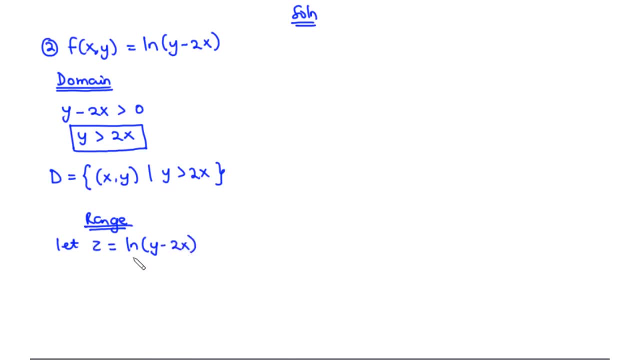 now notice that for the range, we always look at the set of output values of the function. so here what we are going to do is we are going to substitute values of x and then y into this function, having in mind the constraints. constraints or the restriction. okay, so whatever value we select for x, y should be greater. 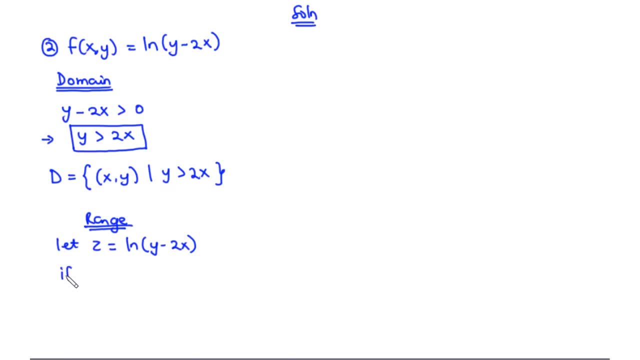 than twice of that value. so let's say, if x is selected to be one, then it means that for y to be greater than two times of x, now two times x or two times one is two. therefore, we can select y to be equal to three. we can select y to be equal to three because three 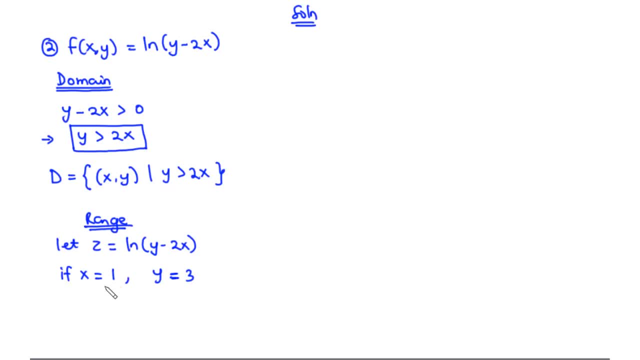 is greater than two times one. good, now let's substitute the values of x and then y into this function. therefore, we have z equals ln of three minus two times one, and that is two, that is two, and therefore we have this to be ln of one. now, ln of one is equal to zero. 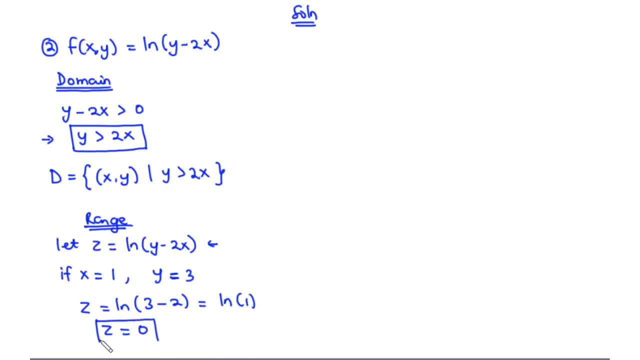 so you realize that here we have a unique function. now, if you split it into two, then you will see that u Michael will smoke to the left side because u m Michael will smoke to the right. so that means we are not only having a relative 感 problem, but we are having other families, having samen before me and other families. 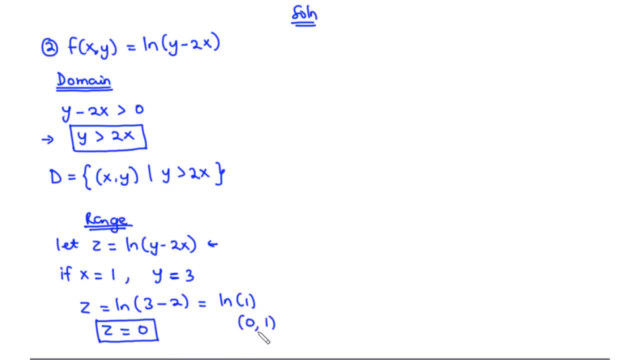 who are instead of and between these two realtions. we have these two puntos, so we are in general the incompatible. so then z is going to be a negative value. so let's say, if you have ln of, let's say 0.5, and so on and so forth, like numbers greater than 0 and then less than 1, you are going to obtain 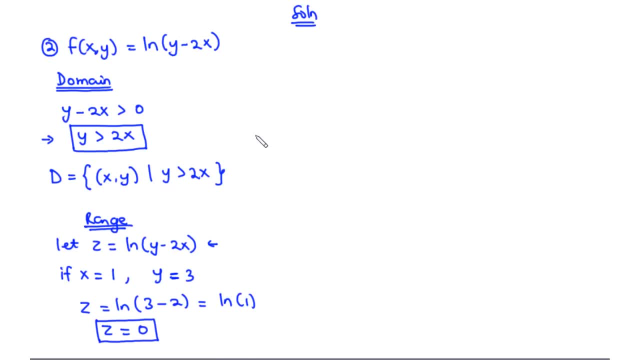 a negative value for z, and then, if you have values greater than 1, you are also going to obtain positive values. now, since we have 0 negative values and then positive values, what this primarily means is that the range is the set of all real numbers, so the range of this function. 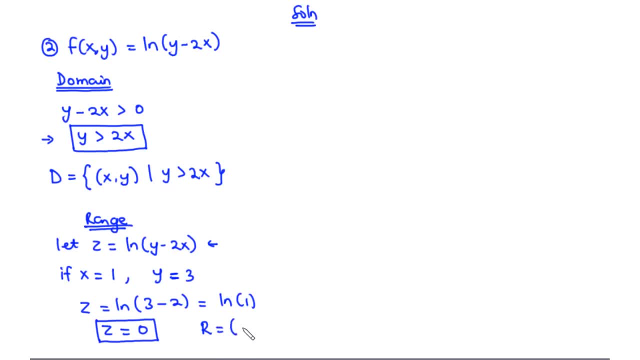 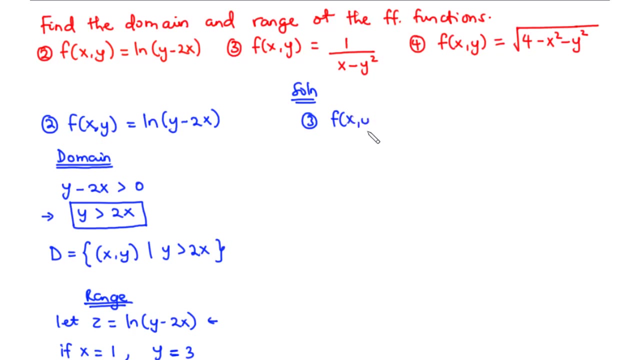 is said to be the set of all real numbers, from negative infinity through to positive infinity. now let's move on to example three. so, for example three, we have f of x comma y, and that is equal to 1 over x minus y square. now this is a. 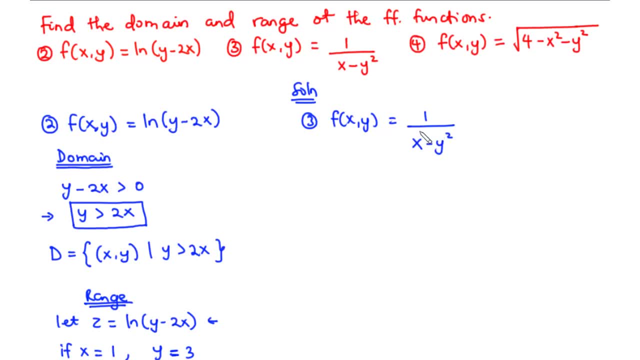 a function. and then you know that for a rational function the denominator is not supposed to be equal to 0. now, if the denominator is 0, it means that the function is undefined. so for the domain, for the domain, the denominator is not supposed to be equal to 0. so for X minus Y, square equal to 0, we have X to be. 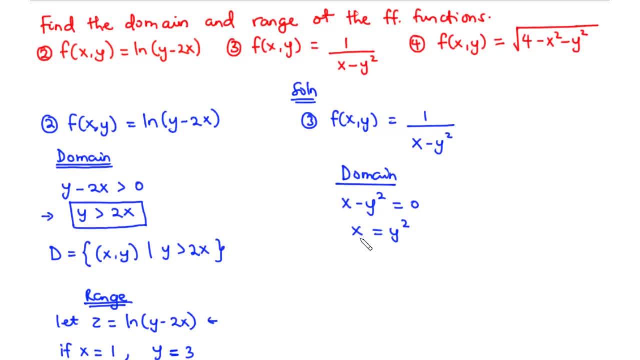 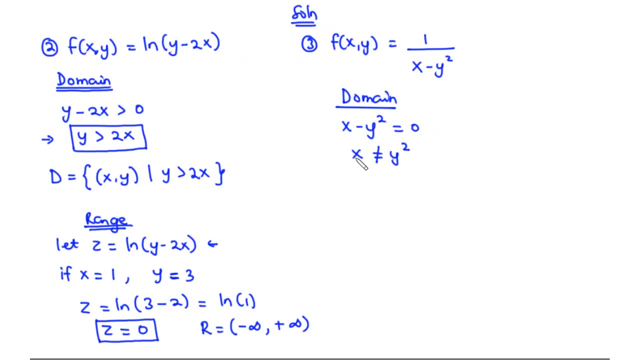 equal to Y square and then notice X is not supposed to be equal to Y square, because if X is equal to Y square, then it means that the denominator goes to 0. so here also we have a restriction, that is, for any value selected for X. it. 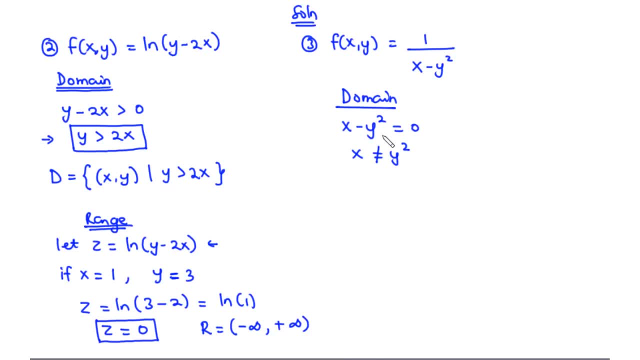 should not be equal to Y squared or X minus Y squared should not, should not be equal to 0. so for the domain, we have the domain to be the set of all grip and lopabi ordered pairs x, comma, y, such that x is not equal to y square, or or the domain is the set of all. 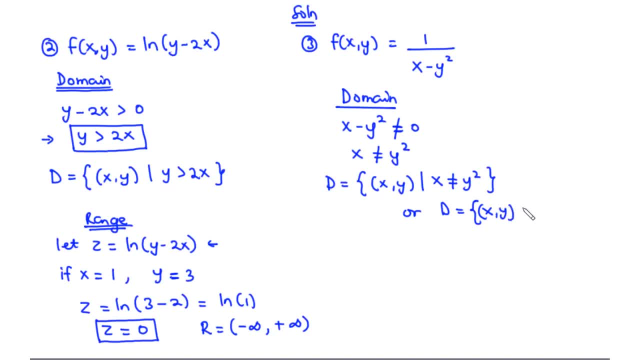 ordered pairs x, comma, y, such that x minus y square is not equal to zero. so any of the two is correct for the domain. now let's move on to the range. let's move on to the range. now for the range. that is a bit dicey, so we want to focus on the output values when we want to talk. 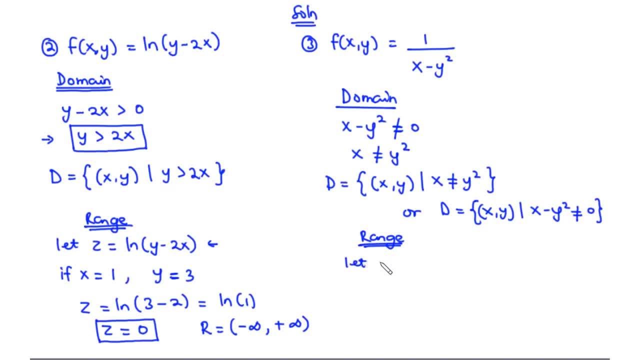 about the range. now for the range. first, we are going to let z. we are going to let, we are going to let z be equal to f of x comma y, so that is 1 over x minus minus y square. okay, so now for this function. first of all, we are going to let y be any arbitrary value. okay. so let's say: 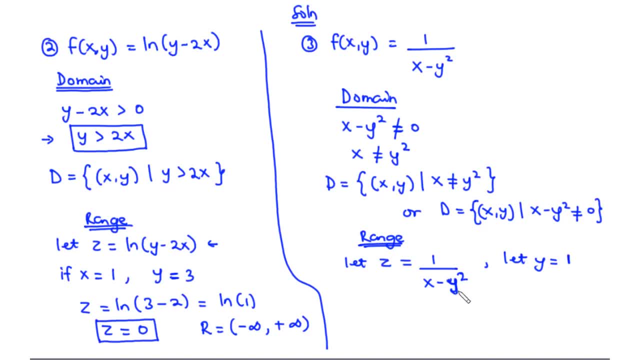 we are going to let y be equal to 1 now. if y is equal to 1 now you can select any other value for y. if y is equal to 1, let's try to find the value of x, or let's try to solve for x. so we are going. 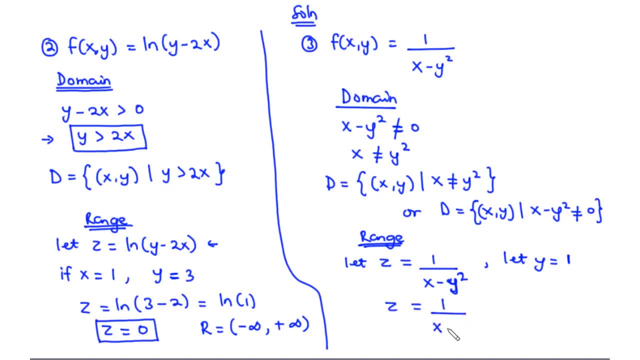 to have: z equals 1 over x minus. now y is equal to 1, so we are going to let y be any arbitrary value. okay, so we are going to let y square or one square is still, it's still 1, so we have 1 over x minus one. 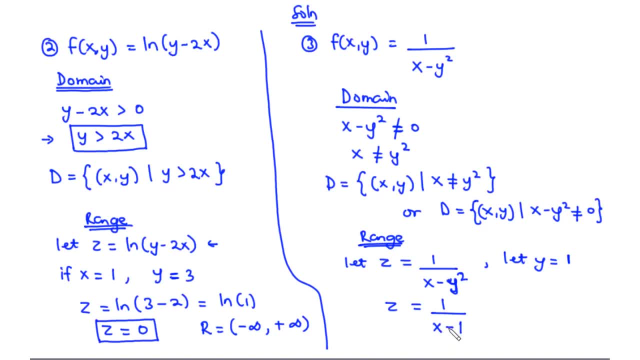 now we want to make x the subject, or we want to solve for x, so we interchange the positions of these two components and then we are going to have x minus 1. okay, we have x minus 1 equals one overぜ. and then we can transpose negative 1 to the right hand side. so at the end you are going to have: 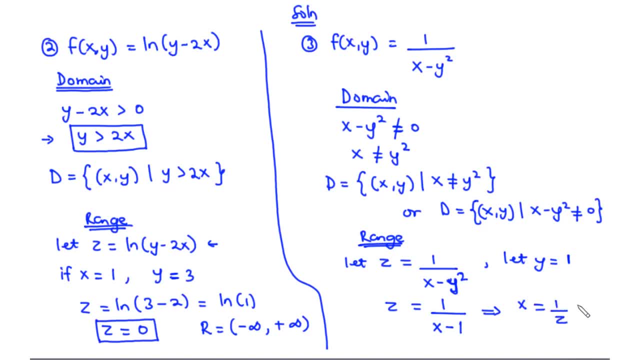 x equals 1 over z plus 1.. So we are going to have an ordered pair x comma y. Okay, So an ordered pair x comma y, which is for x. we have 1 over z plus 1. comma y is 1.. So for y equals 1, and then for any value: 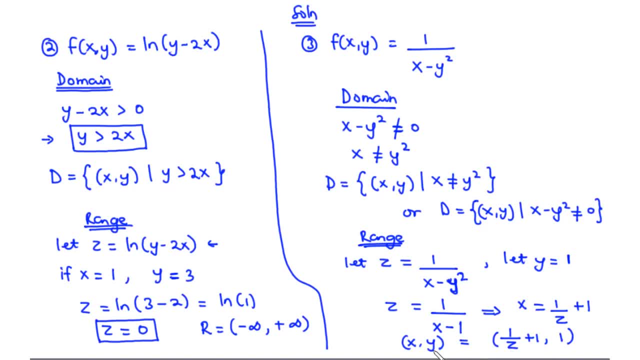 we select for z, we are going to have an ordered pair, x comma y, as 1 over z plus 1 comma 1.. Now x here becomes defined if, and only if, the value of z is not equal to 0.. Now, so long as z is equal, 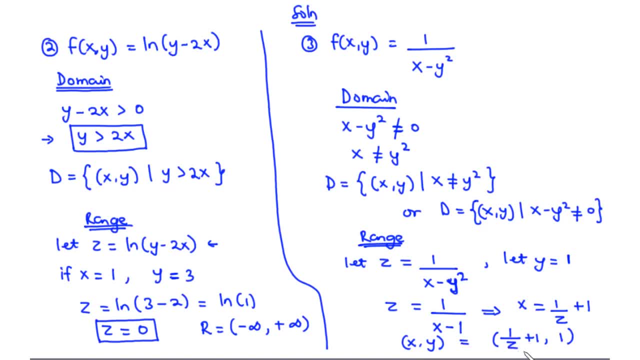 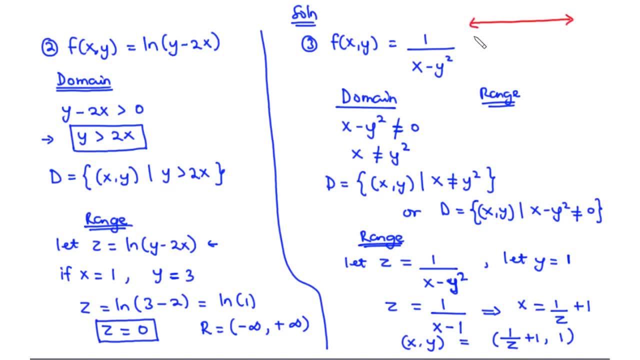 on the real number line. we have this to be negative infinity and then this to be positive infinity, and then we have 0 in here Now, because 0 is not included in the set. we are going to have 0 in here Now, because 0 is not included in the set. we are going to have. 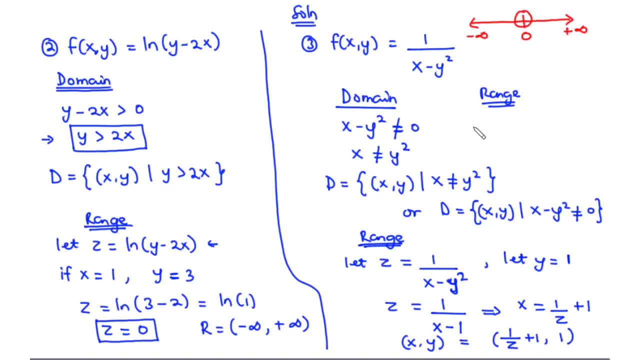 an open circle. Therefore you can represent this as: the range is the open interval from negative infinity to 0. So 0 is not part of the set union, the open interval from 0 to positive infinity. So this is the range of this function. 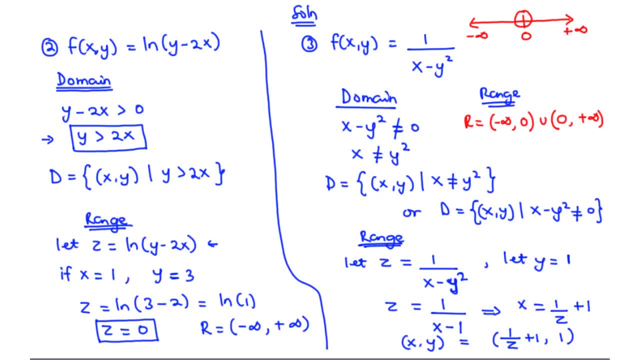 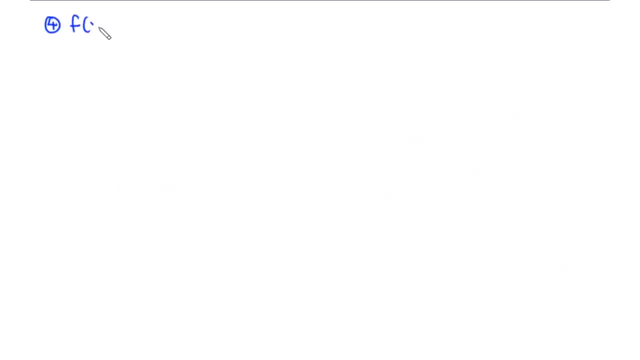 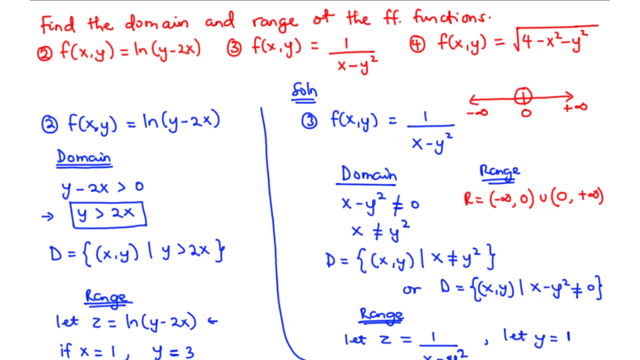 So at this point you realize that there is no defined approach in finding the range of a function. It mostly depends on the type of function you are dealing with at the moment. Now let's move on to example 4.. So for example 4, we have the function f of x, y, and that is equal to the square root of 4 minus x squared, minus y squared. 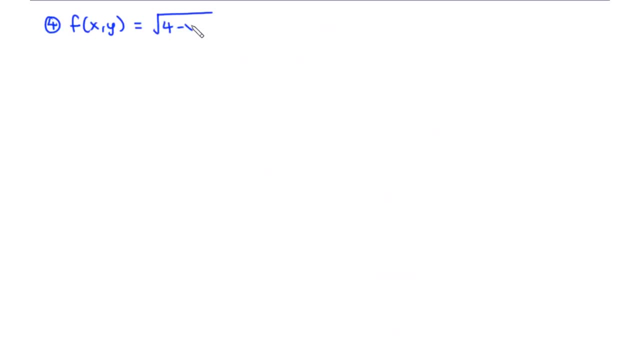 So the square root of 4 minus x squared minus y squared. So first let's try to find the domain. So for the domain, that is the set of all ordered input values that makes the function defined. So this is a square root function. 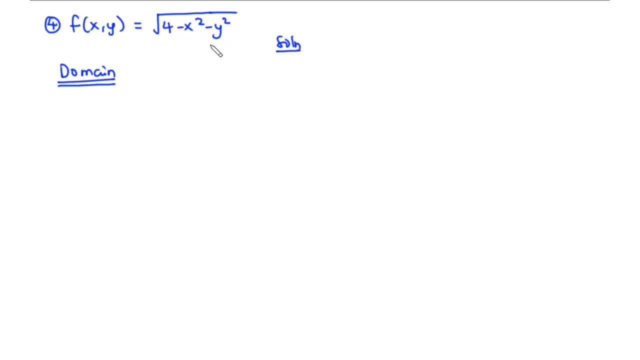 Now, to make this function defined, what we need to do is to ensure that the expression under the square root should be either 0 or greater than 0. So for this to be valid, it means that the value under the square root should be greater than or equal to 0.. 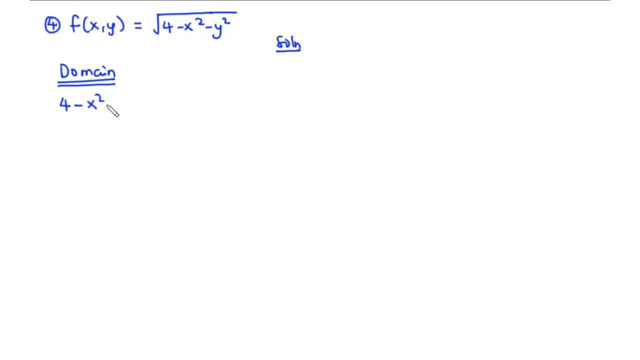 So we are going to set 4 minus x, So we have 4 minus x squared, minus y squared greater than or equal to 0.. And then we can transpose negative x squared negative y squared, to the right hand side, So we have 4 greater than or equal to x squared plus y squared. 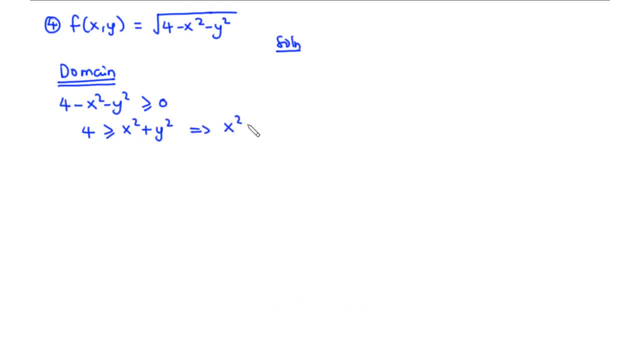 And then we can also represent this as: x squared plus y squared is less than or equal to 4.. I mean, they are the same. Therefore, we have the domain of the function to be The set of all ordered pairs, x, comma, y, such that x squared plus y squared should be less than or equal to 4.. 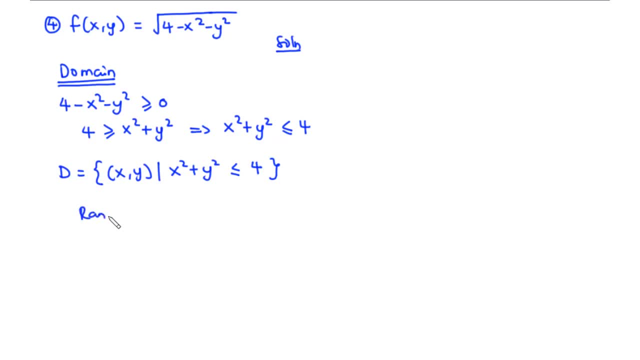 This is the domain of the function. Quickly, let's move on to the range. Now to find the range, we are always looking at the set of all output values. Now for the range. we let z be equal to f of x. 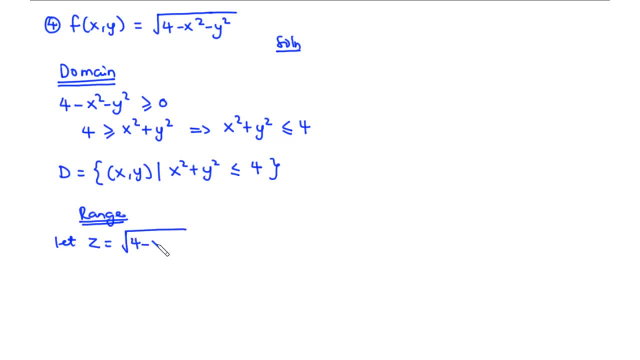 And that is the square root of 4 minus x squared minus y squared. Now, since this is a square root function, the smallest value we are going to obtain for z is when z is equal to 0. Because the value or the expression under the square root cannot be a negative value. 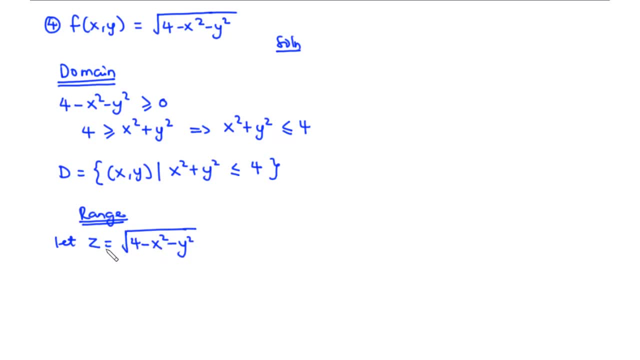 And so the smallest value we are going to obtain for z is when z is equal to 0.. So let's say, the smallest value, the smallest value of z is equal to 0. so again, how do we find the highest value? how do we find the highest value? 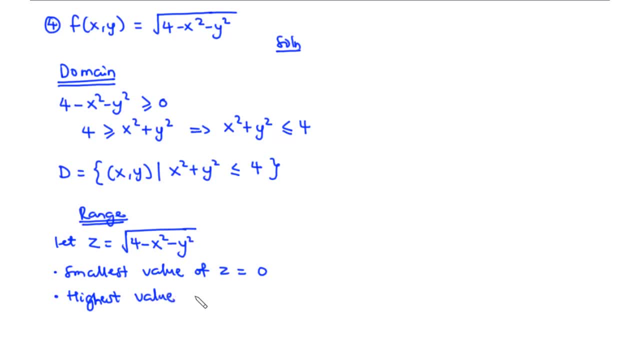 the highest value, the highest value of z. so for the highest value, to obtain the highest value, what comes in mind is we need to select very small values of x and then y, so that the expression or the value under the square root can become something big. 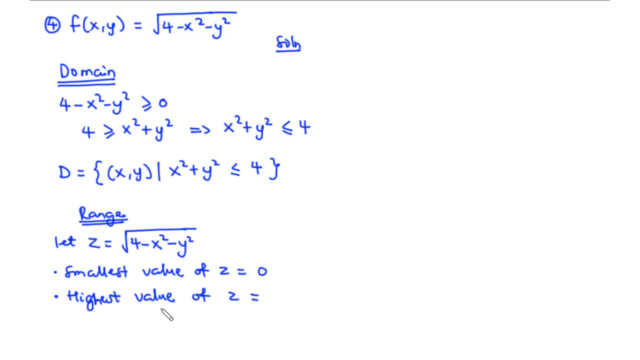 and then that will make us find the highest value of z. now, what I mean here is that, for instance, let's say you have the square root of 10 minus x squared. now if you want to get the maximum value, you need to ensure that x is equal to 0.